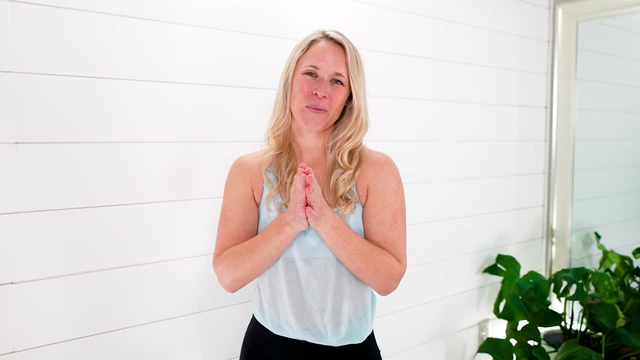 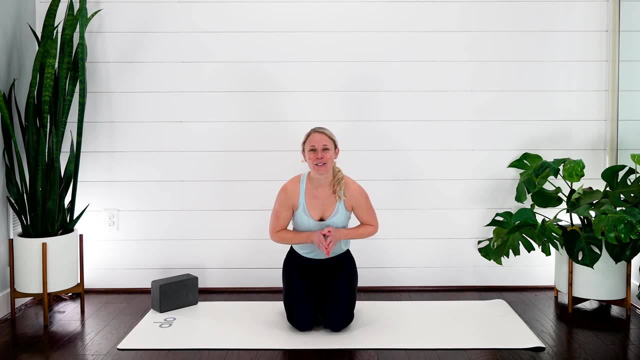 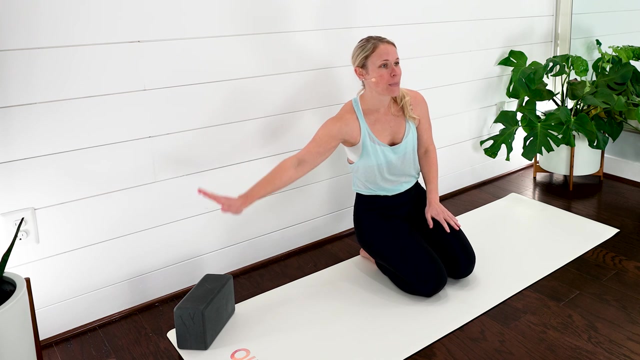 Go, grab your mats and let's do this. All right, let's loosen up those pelvic floor muscles. If you've noticed that you hold a lot of tension or tightness or those hypertonic muscles, we're going to go over the perfect exercises to really lengthen and relax those pelvic floor muscles. If you happen to have a. 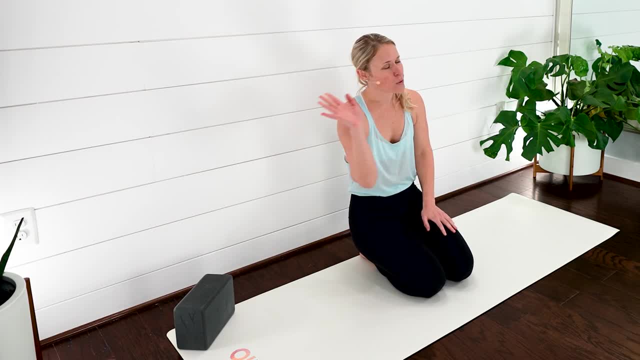 yoga block. go ahead and grab that. If you don't, no worries, I've got you covered, So let's get started Coming in. we're going to be going over exercises that help relax and lengthen our pelvic floor muscles. If you've noticed that you hold a lot of tension or tightness, or those hypertonic. 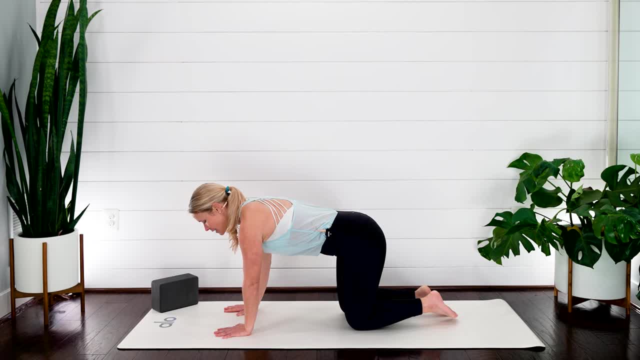 muscles. we're going to go over exercises that help relax those pelvic floor muscles, If you've noticed that you hold a lot of tension or tightness or those hypertonic muscles. we're going to go into tabletop position, So those hands underneath your shoulders, knees, hip distance apart. 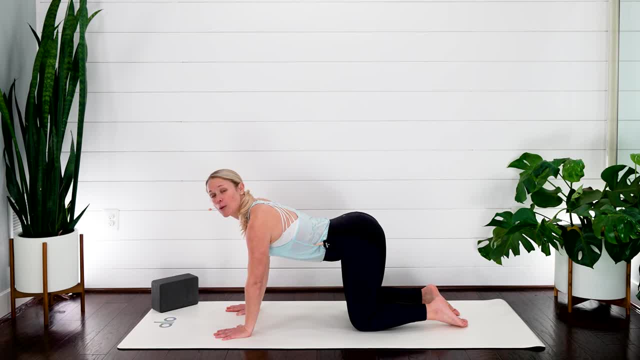 and we're going to take a nice gentle breath in, Lift your tailbone, lift your head, And I want you to think of your sit bones spreading apart and just this opening, relaxing of those pelvic floor muscles, kind of like a blossoming. And then we're going to exhale, round everything out, pull the. 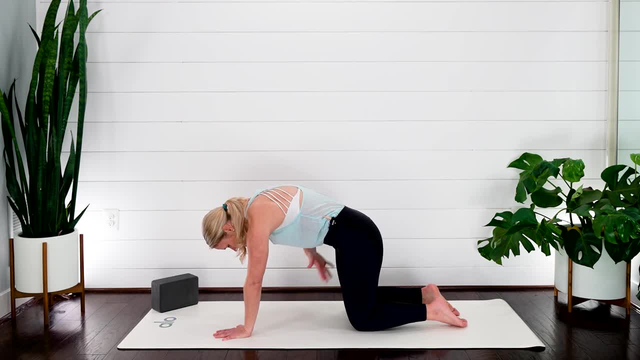 chin towards your chest, tuck your tailbone underneath, and you might feel this gentle pulling that lower abdomen. and then inhale. lift your head, tailbone comes up, spread those sit bones again, really emphasizing on the m: uh, inhale part good, exhale, round it out. 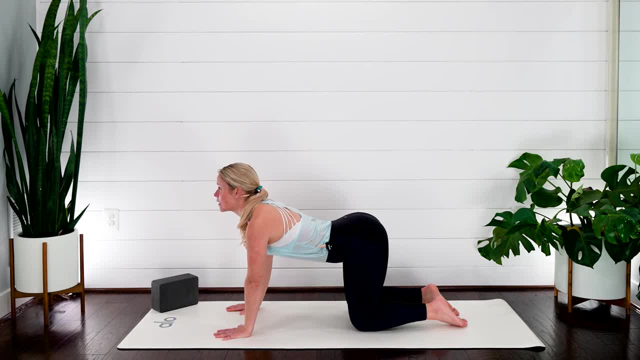 nice and slow movements. inhale, lift your head, lift the tailbone. good, this time we're going to add on when we curl and round underneath. just take those toes and gently curl your toes underneath. pull your chin towards your chest, so our feet are also connected to our pelvic floor. inhale, lift the chest. 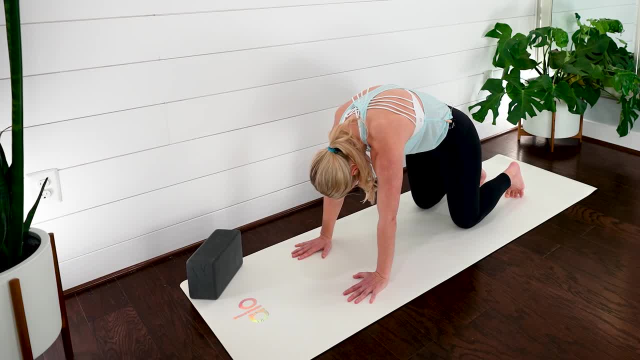 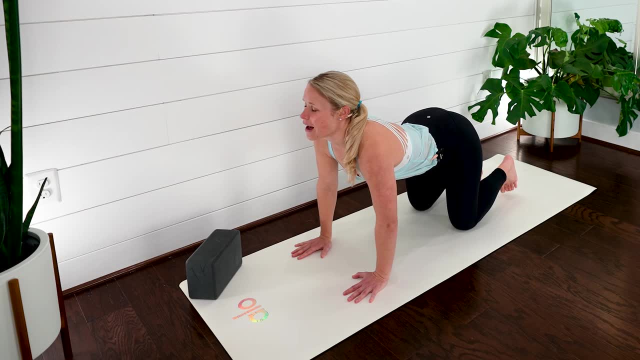 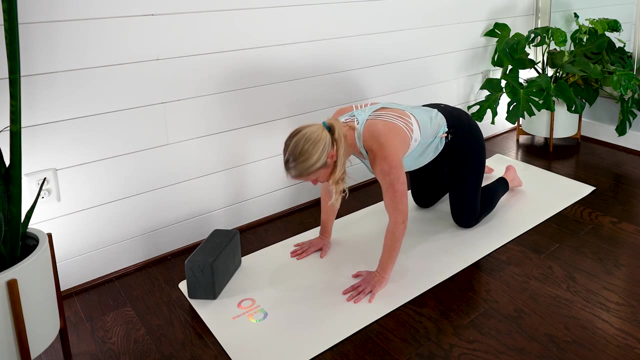 and then round it out. curl your toes, tuck your tailbone, just a gentle stretch in the bottom of those feet. inhale, lift, exhale, round out and our breath. we're trying to send our breath as far down the back as we can, so really trying to get into the 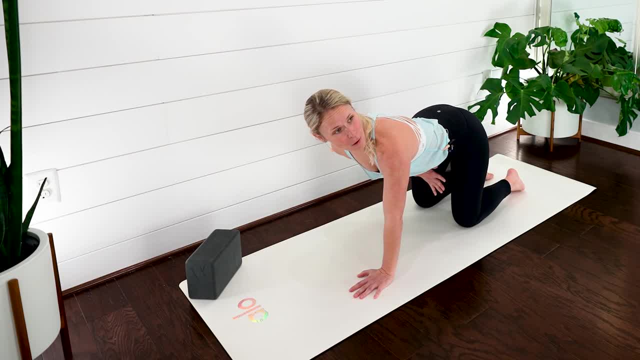 body and stretch those core muscles out, strength the core muscles that we're working on. so we're really trying to get into the back of the body as much as we can. so really trying to get into the of the ribcage, that diaphragm sending our breath all the way down to the 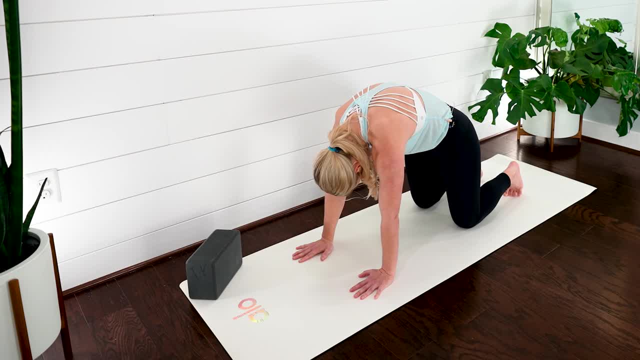 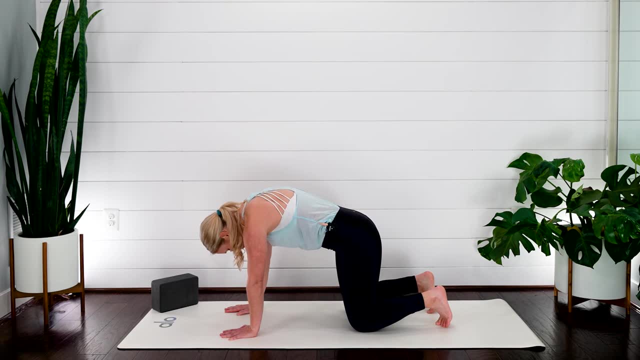 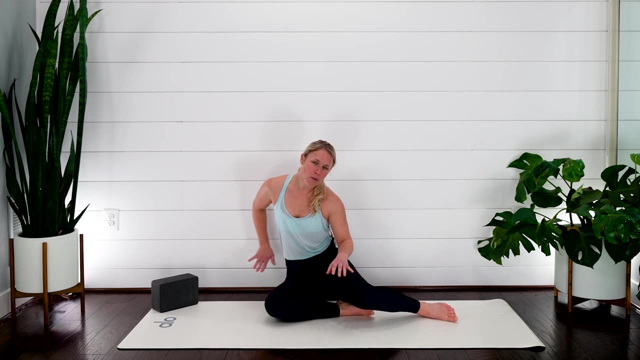 pelvic floor muscles. nice job one more time: inhale, lift, exhale round it out and then come to seated position. if you have a wall or something up behind you, you can go sit next to that. if not, no worries, we're gonna start bringing our feet in two cobbler's pose. the soles of the feet are coming together and just. 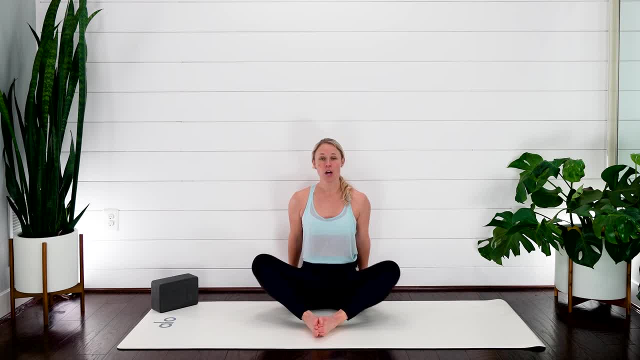 start by taking your hands and placing your hands behind you. you want to think of your knees, pushing those knees down towards the ground and you're opening through the front of your chest, maybe just kind of wiggling from side to side, pushing one side down, then the other, and just noticing any tightness that you're. 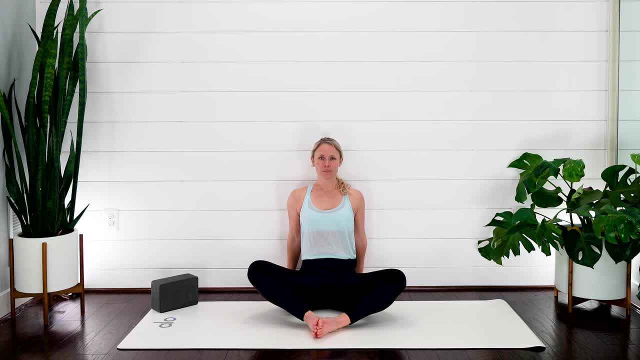 feeling in those inner thighs or in your hips. take a nice gentle breath in. that breath is going all the way down- exhale, let it relax good. another nice gentle breath in- exhale, let that go good. now, if you don't have a wall behind you, you're gonna go ahead and grab hold of those ankles. stay lifted through the. 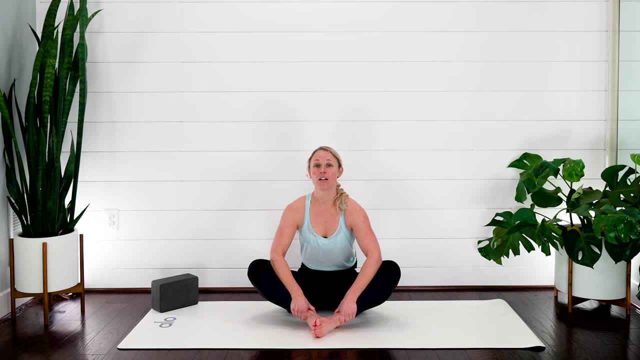 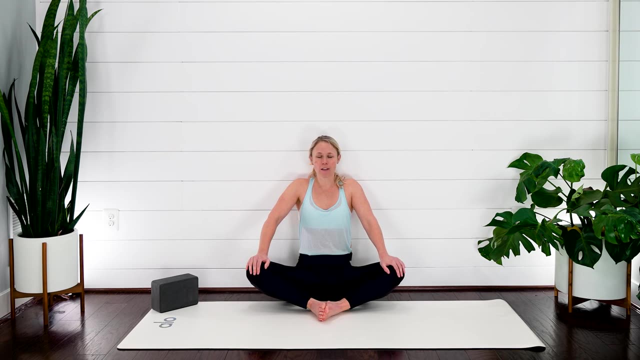 chest and you can use your elbows to push those knees down towards the ground, trying to hinge forward without coming into this rounded tucking our tailbone underneath. if you've got that wall behind, you can kind of scoot up against it, bring those feet in and then those arms come to your inner thighs and just gently push the. 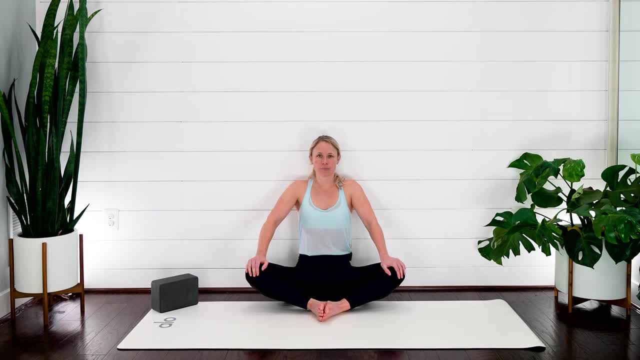 thighs down towards the ground, opening up, and we're really working on the breath. the breath is the key to helping lengthen those pelvic floor muscles. so when we breathe in, we're sending our breath out to the sides of our ribcage. that diaphragm comes all the way down and we just think of opening, spreading. 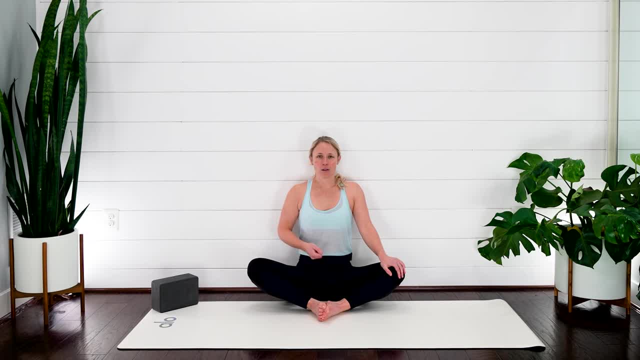 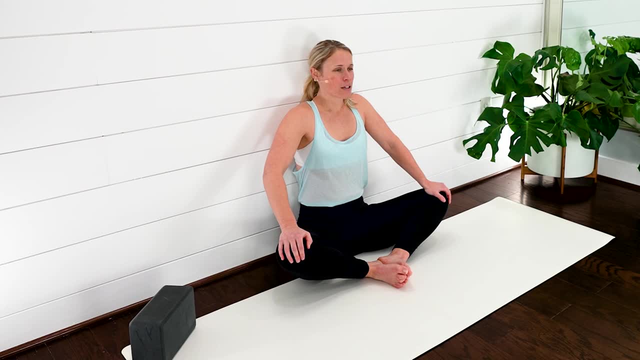 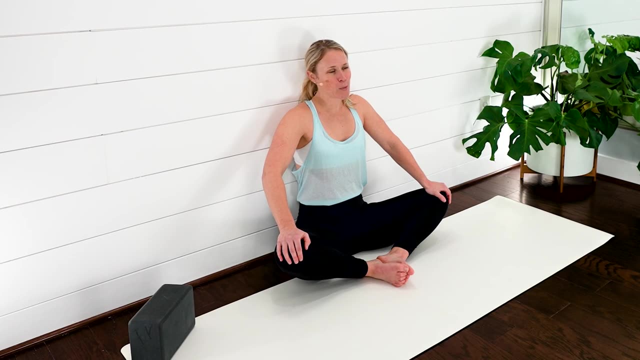 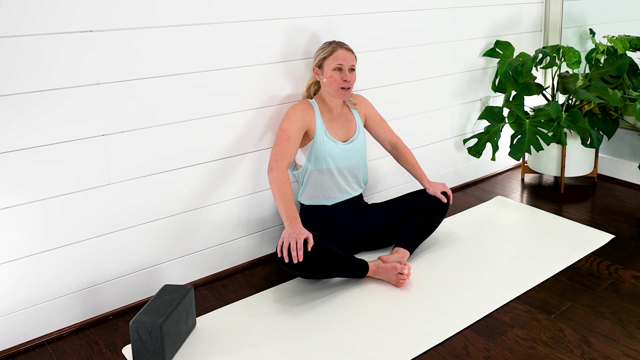 apart and then exhale. it comes back up. inhale this softening and lengthening, just being nice and gentle, trying to open up those inner thighs. so making sure we have some good mobility and a range of motion in our hips is really important to helping relax the pelvic floor, because one of our hip muscles 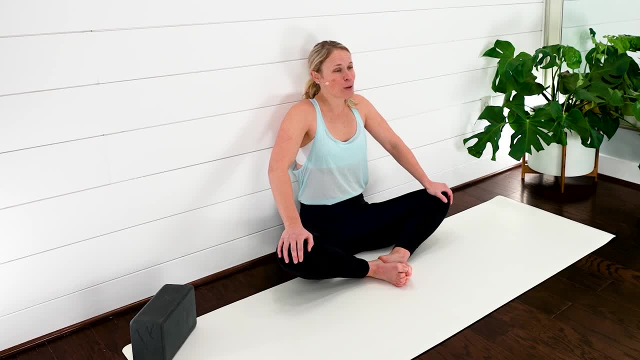 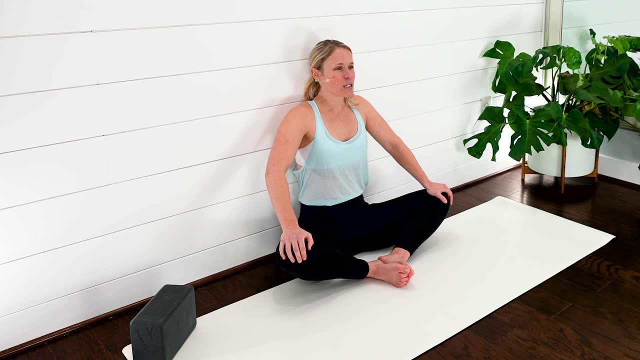 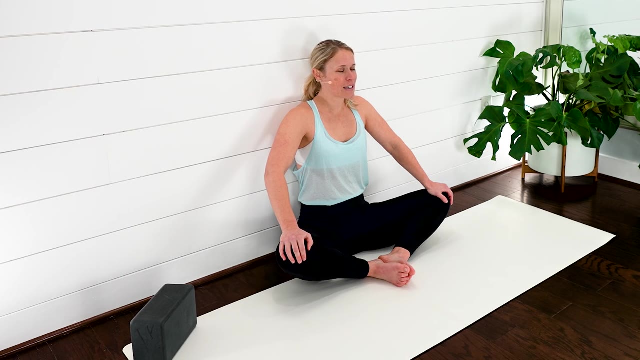 it's called. your obturator internus attaches into our pelvic floor, so it's a great way to relax the pelvic floor. so if the hips are tight, that muscles also gonna pull on our pelvic floor. let's just stay here for a couple more gentle breaths, in seeing if you can soften a little bit each breath, being careful the 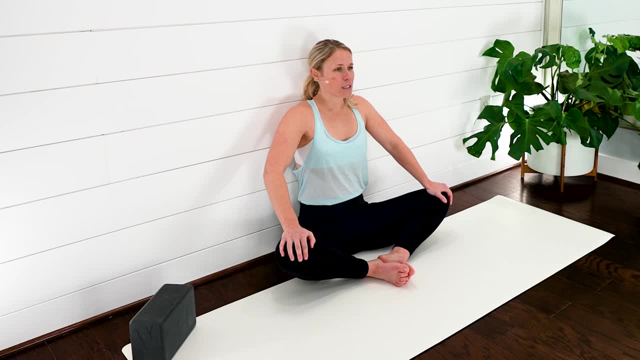 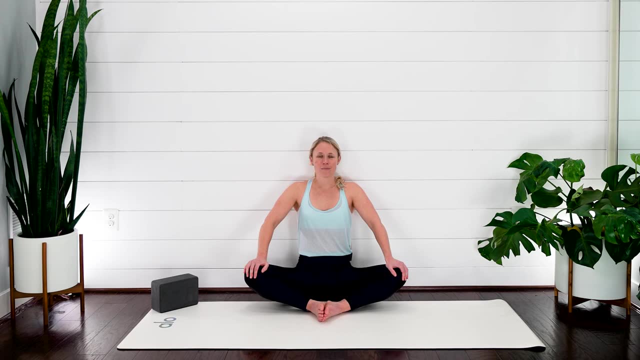 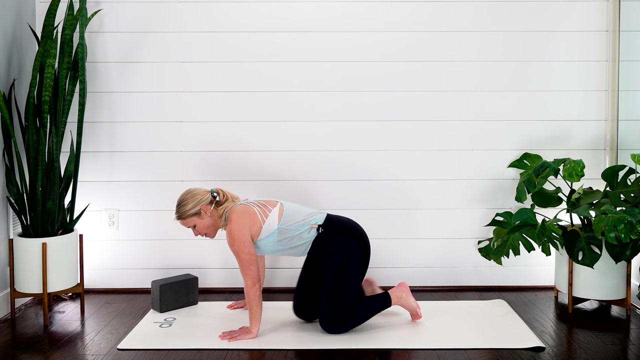 breath isn't coming up or staying up into our chest. nice job, we've got one more gentle breath in here. exhale, let that go good, and then slowly bring those legs come back up, and then we're gonna come back onto our hands and knees into that tabletop position. 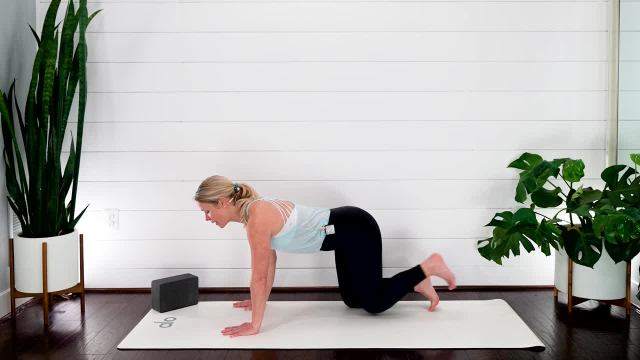 you're gonna take your left leg, send your left leg straight behind you and bring it over towards the right hand side, curl your toes underneath and just turn to take a gentle, peak, feel, a gentle, stretch down that left hand side and then you're gonna lift the leg up, exhale, bring the knee to that elbow and then 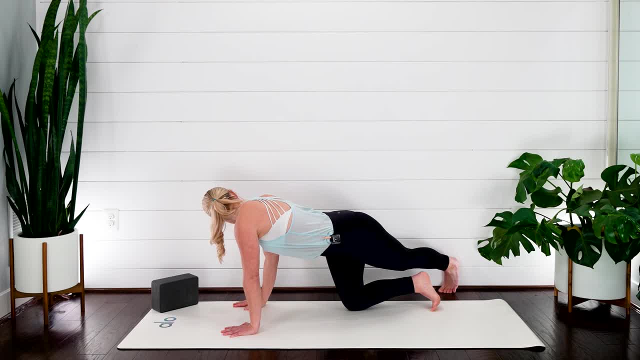 send the leg straight back behind, over towards the right hand side, and then maybe you just do a couple little pulses reaching back, turn to look at it, feel to stretch down that left side, lift the leg, exhale, hug that knee in and then take the leg back one more time, those little pulses going back. good, 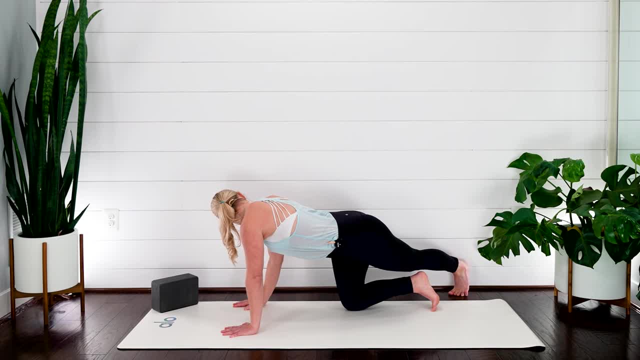 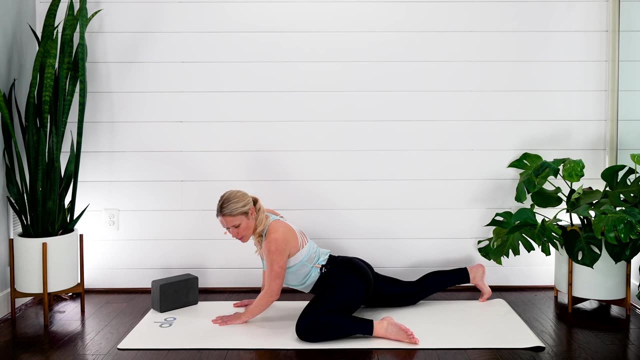 one more time, those little pulses going back. good, and then bring the leg, come back up, exhale, bring that knee in towards your elbow and then we're going to take the leg lower, that leg down. show you two options here. so you can keep scooting down, so you've got one leg coming into. 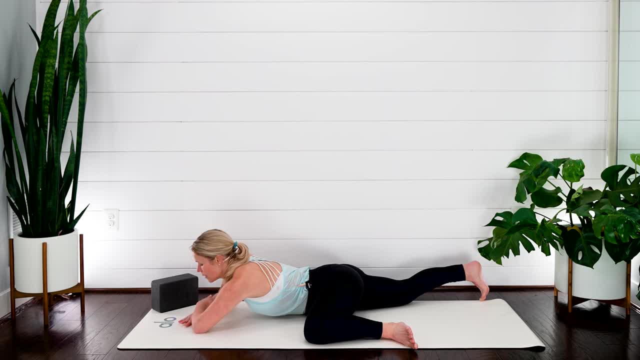 this frog pose and we're thinking of pushing the hips towards the ground. you're gonna rest your forehead down on those elbows. I'm gonna stay up, just so you can hear me. we're trying to have a nice inner thigh stretch. one might feel awesome and you want to stay there if you wanted to do both of them, both knees. 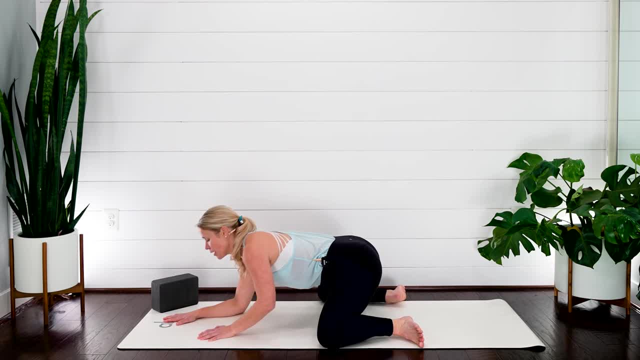 mat distance apart. sink those hips back, breathing into it the same thing, thinking of spreading the sit bones apart, opening up the hips, the breath going all the way down. see how far down you can get it into the back of the rib cage. nice, gentle breath in exhale. let it go. 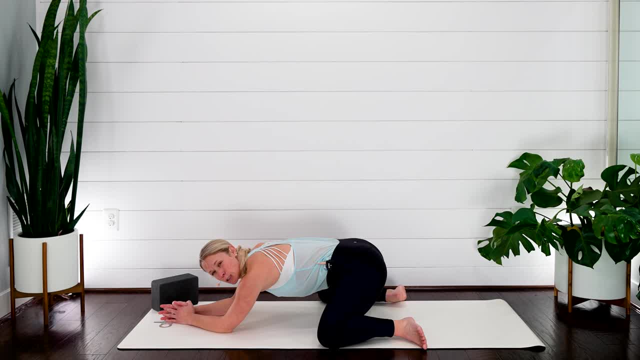 and then we're going to take a deep breath in. and then we're going to take a deep breath in, and then we're going to take a deep breath in and just notice where you're, just notice where you're feeling any tension or tightness. gentle breath in. 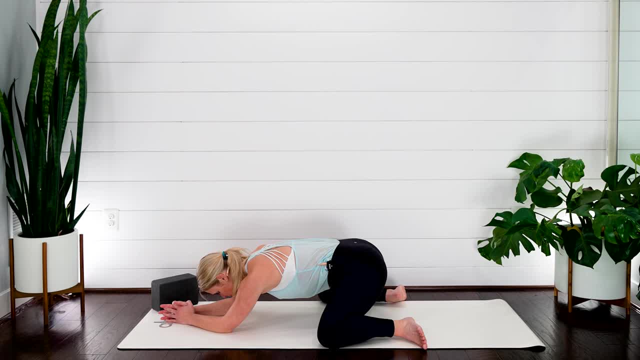 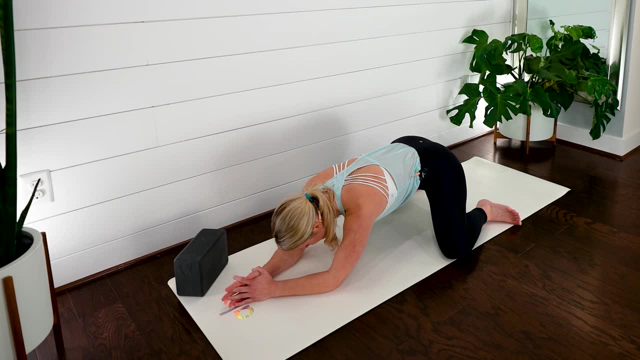 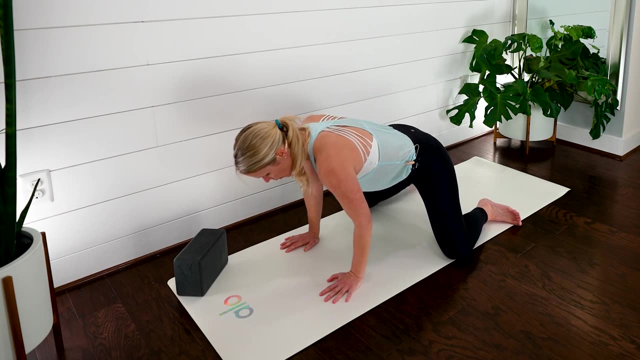 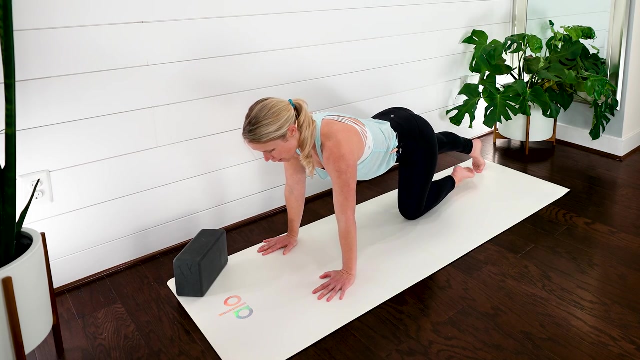 exhale soften. let it go. take one more breath in here and then pull yourself, come back up. we're gonna scoot those knees back underneath us. coming in a tabletop this time, coming in a tabletop this time. that right leg goes straight back behind. press into the top of your left foot. 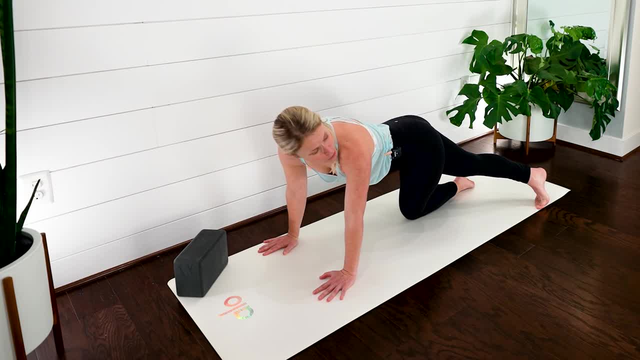 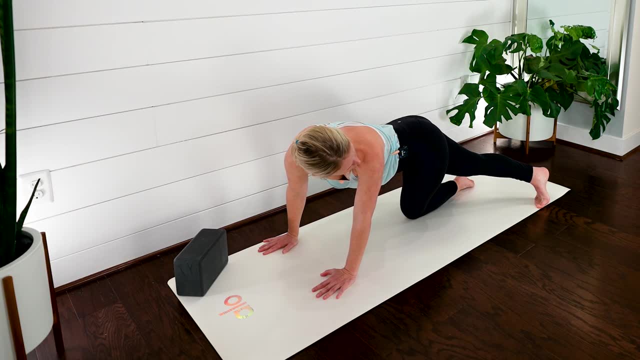 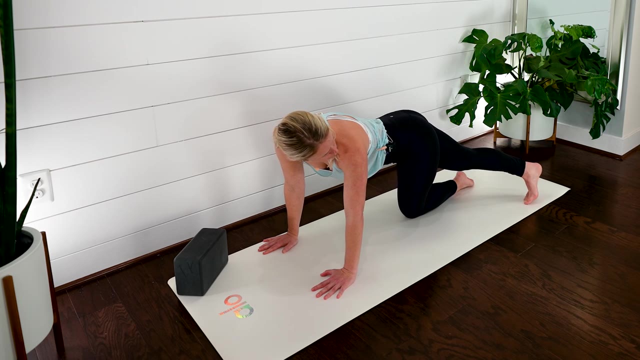 lift the leg up and over towards the left hand side, turn to take a peek press through the back heel, gentle push of the arms over towards the right hand side and then bring the leg up, exhale knee to elbow, send the leg back behind, press through the heel. maybe you do a little pulses pressing back, little pulses with. 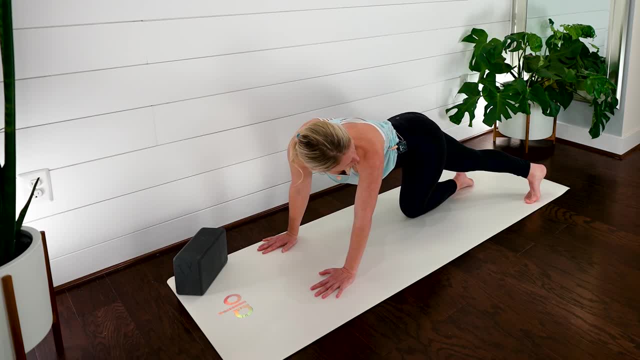 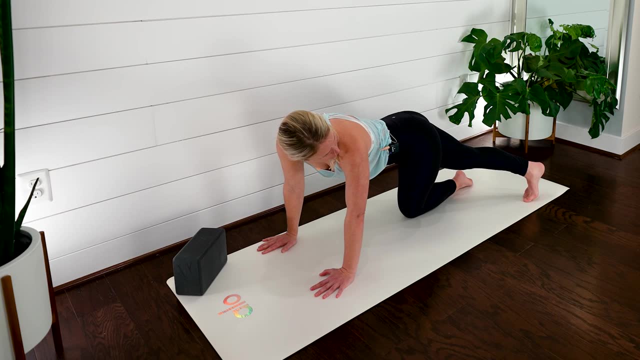 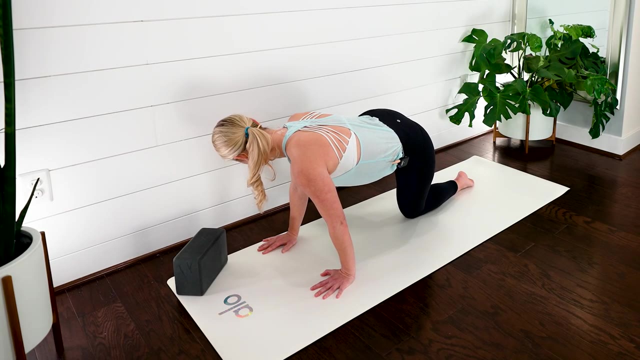 the hands over towards the right hand side just to feel the stretch down the right hand side. lift it up, exhale, turn, take a peek, send the leg back. last one stretch through the back heel. a nice gentle breath in exhale, bring elbow to knee and then option so you lower that right knee down, you can sink your left. 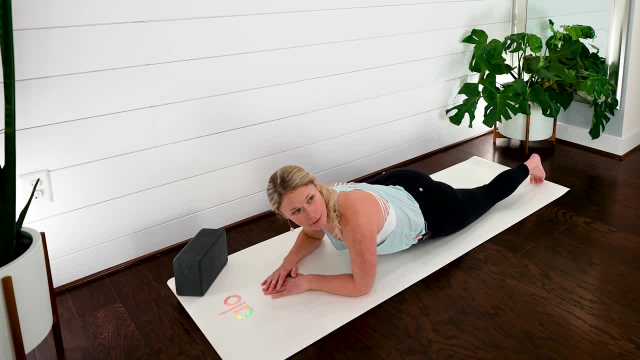 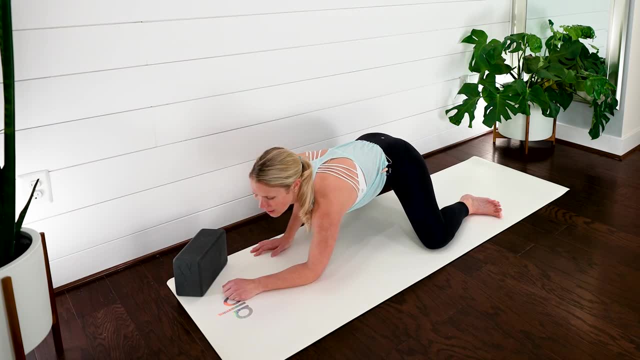 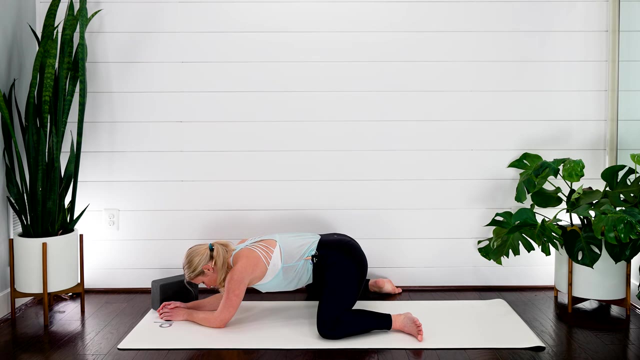 leg, bring it back, pushing that knee down towards the ground, opening up inner thigh. or, if you want to come back into both knees out towards the side and then sink those hips back. gentle breath: in each breath you try to soften just a little bit more. think of 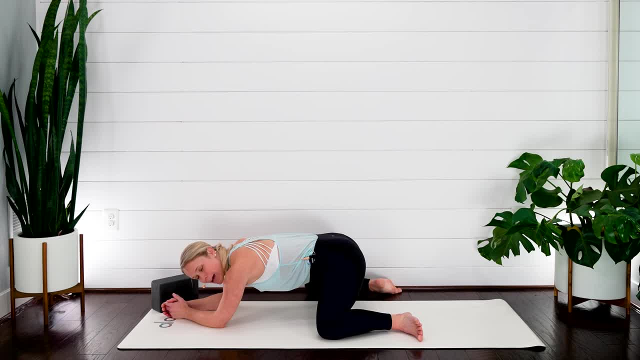 pelvic floor muscles, so from your pubic bone all the way back to that sit bones spreading out. can you notice if you're holding your breath out just a little bit more, you're? your breath is changing, really sending it out to the sides of our rib cage. 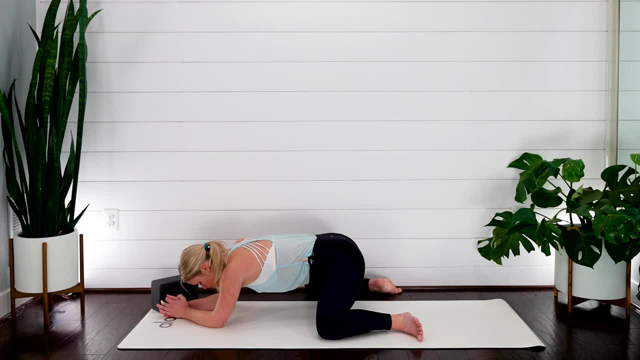 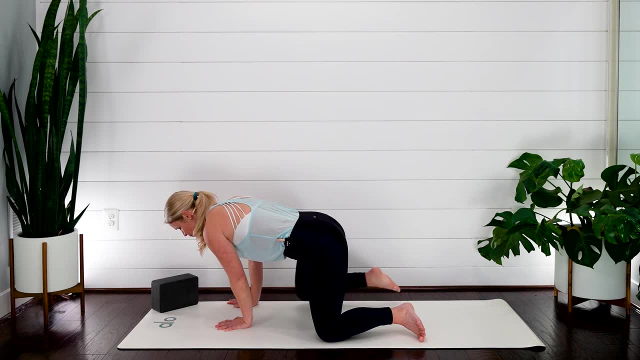 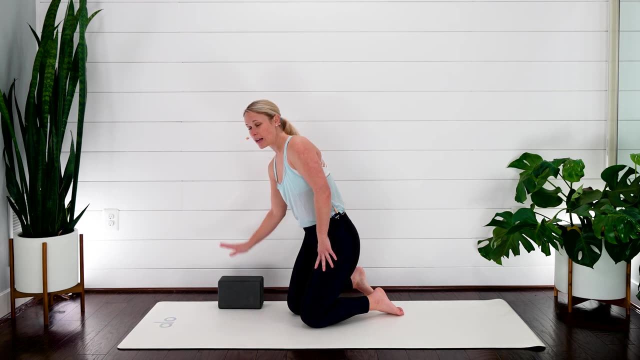 Awesome job. One more breath here, Exhale, let it all go. Good, Come all the way back up. So this next one. we're going to come into a squat position, So if you do have a wall nearby, maybe you choose to use that. If you've got your yoga block, you can use some pillows. 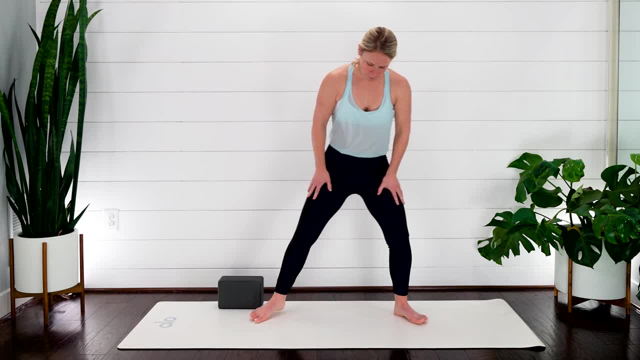 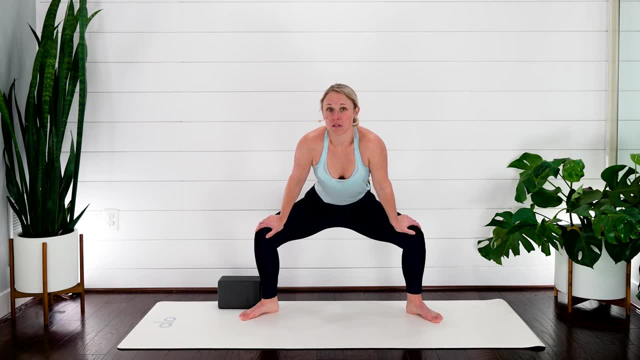 You could also do this in a chair, but we're going to move our feet so they are a little wider than hip distance apart, And then we're going to sink our hips down. You might choose to stay here and kind of push your hands into your thighs opening up. Maybe you choose to. 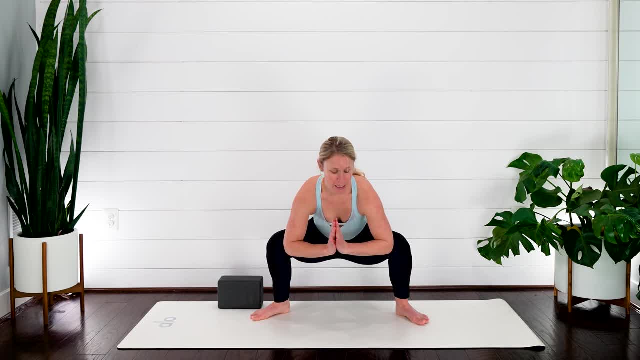 sink the hips all the way down, bring your elbows in towards your inner thighs and you're pushing out, lifting the chest, Trying to open up. And then you can also use that yoga block if you want to just sit on the yoga block and work on lifting up, And the same thing you kind of back up against the wall for. 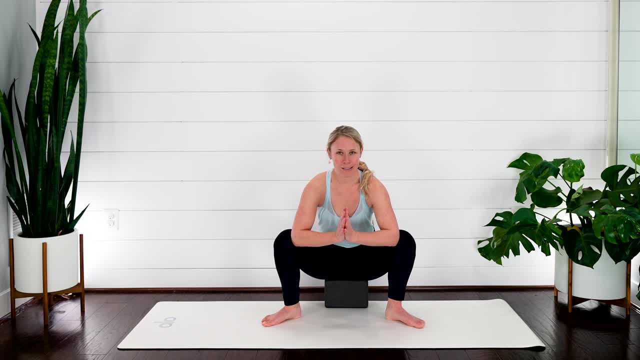 a little bit of support coming into your squat. So find what your body is needing. You can play with the different ones. Our goal is to open up the hips and send the breath down to relax those pelvic floor muscles. So very gentle breaths. 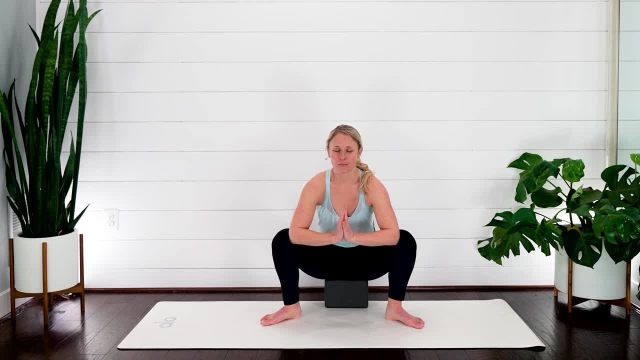 And then exhale, letting it go And just see if you can keep softening, opening up a little bit more. Good, Keep trying to lift the chest, lift that tailbone Pressing into the feet, And then check, can you spread your toes, making sure our feet are nice and relaxed. It's a great way to help relax. 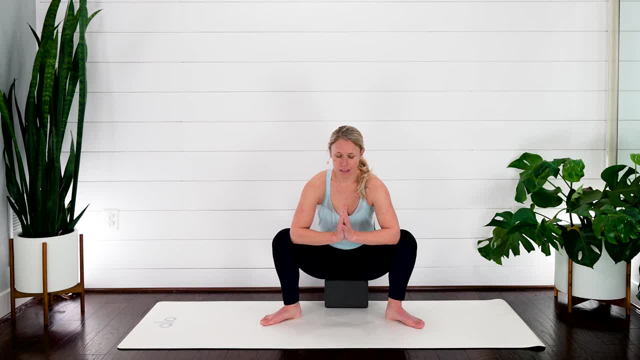 the pelvic floor muscles. Gentle breath in Exhale, let it go. If you want to know more about relaxing your feet, you can go ahead and check out this video up here. Nice, gentle breath in Exhale, let it go. We're just 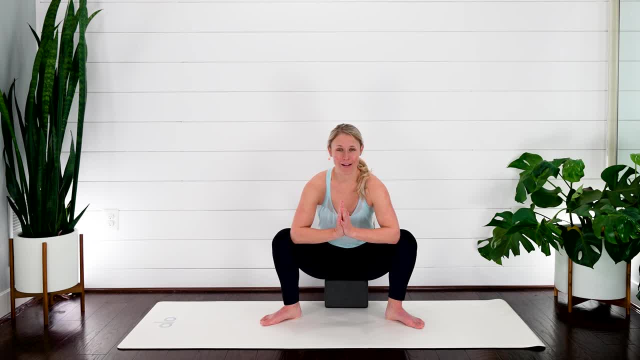 going to hold here two rounds, inhaling for four and exhaling for four. On your next inhale, we have four, three, two one. Exhale four, three, two one. Inhale four, three, two one. Exhale four, three, two. one. 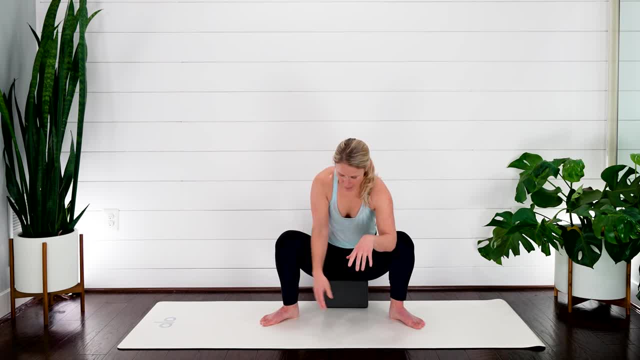 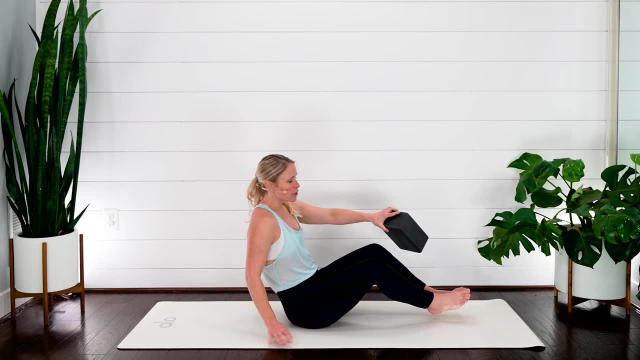 Awesome job. If you want to stand back up, maybe take that block out. We've got one more. This last one is like my all-time favorite: Come down onto your back. If you've got your block, bring that with you. 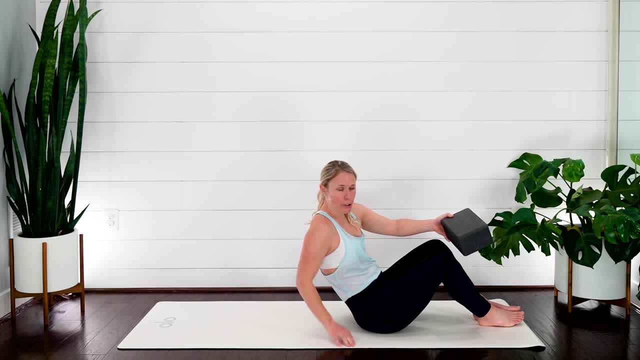 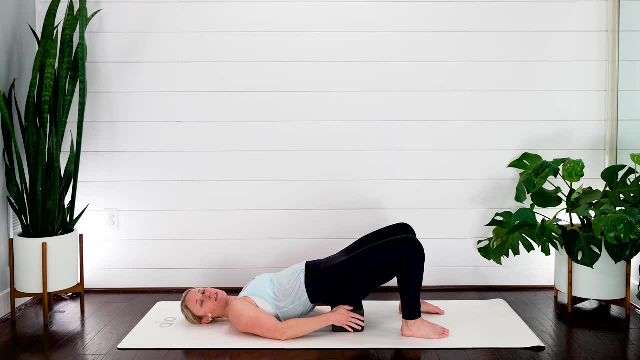 If you don't, you could grab a couple of pillows or also roll your yoga mat up. We're going to come all the way down onto our backs and then just lift those hips up, Take the block or whatever you've got, and put it underneath your low back, So just below belt line area, And then, once you've got, 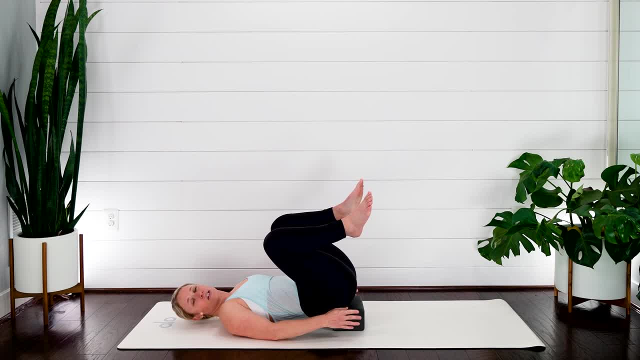 that there you're going to bring your knees in towards your chest and it should feel very supportive, Like you can just kind of hang out here And then we're going to take our hands to the tops of our shins And just gently pull those knees apart, Feel a gentle stretch And, as you're inhaling, send the. 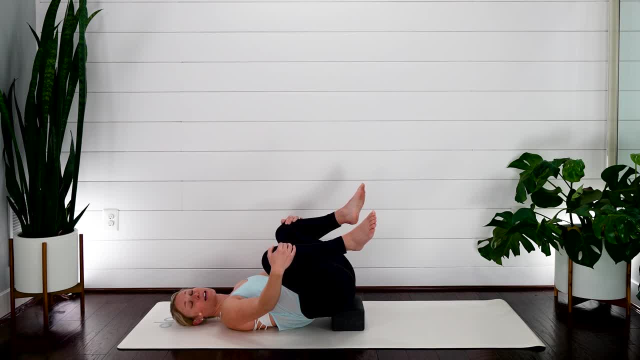 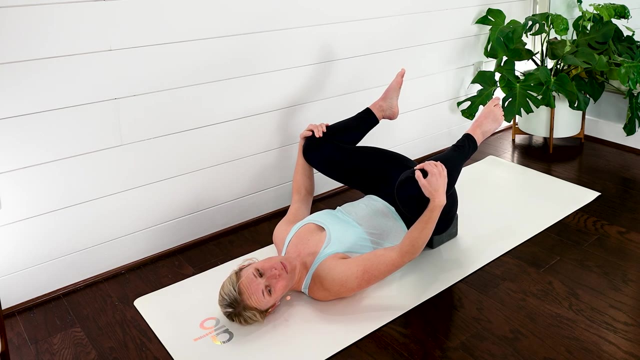 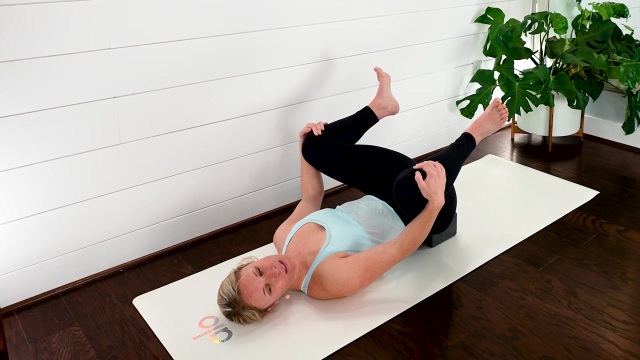 breath down, Exhale, let it go. Maybe you do a little rocking from side to side, But just very gentle. Maybe you find that all of these exercises- or maybe there's one in particular that you can really feel that pelvic floor relaxing with, You can do it throughout your day, Maybe before or 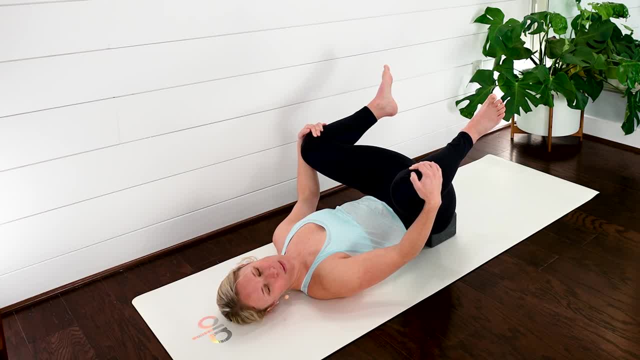 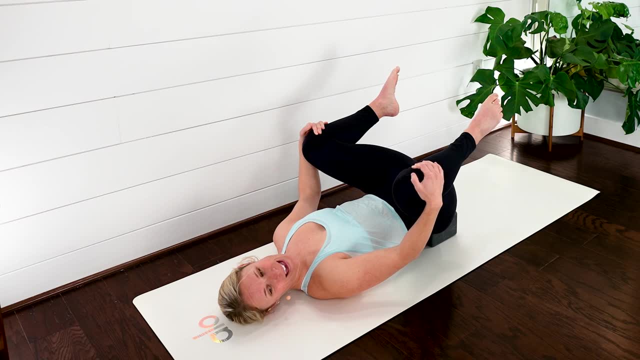 after your workout is great. It's just a great way to help relax and loosen up pelvic floor muscles. We think of stretching other muscles, but not necessarily our pelvic floor ones- And then you'll start to notice the difference as you continue with your breath. Keep up with the 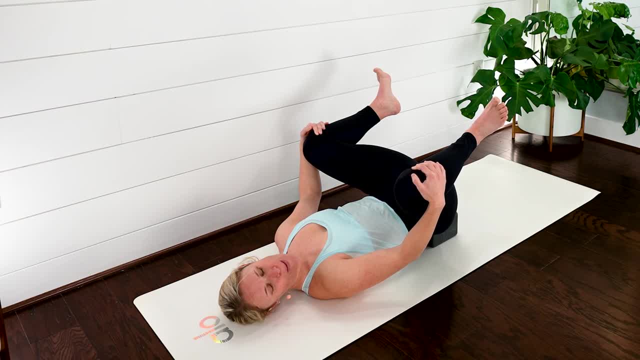 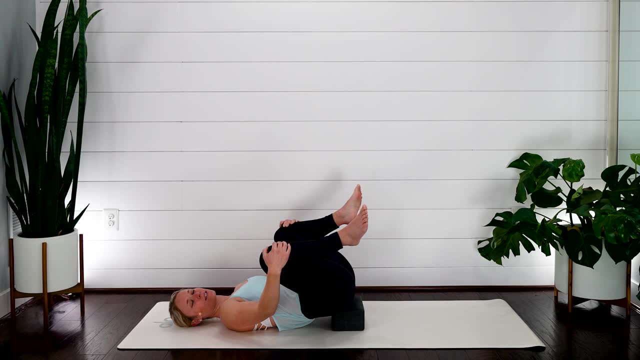 consistency of a regular stretching program to help loosen them up, And you'll notice that change. Here we are Good. Let's take one more breath in hereе. Of course, if this one feels really good, feel free to stay here a little bit longer.